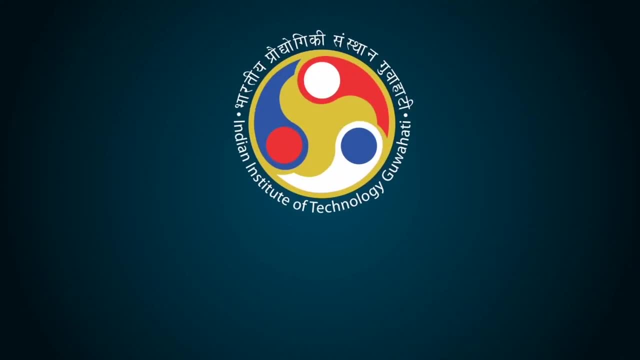 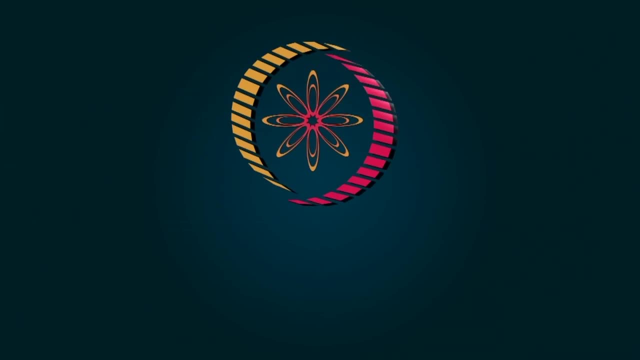 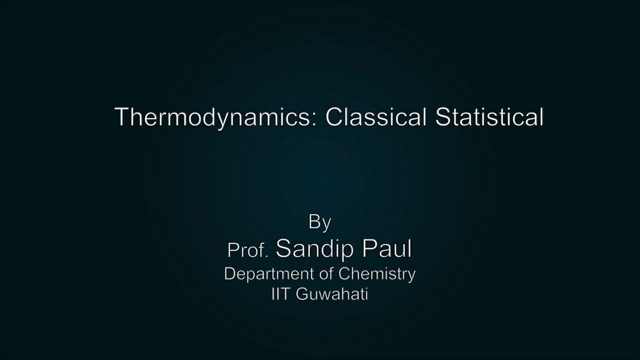 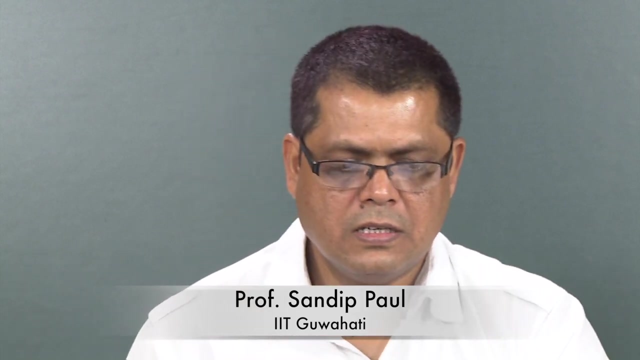 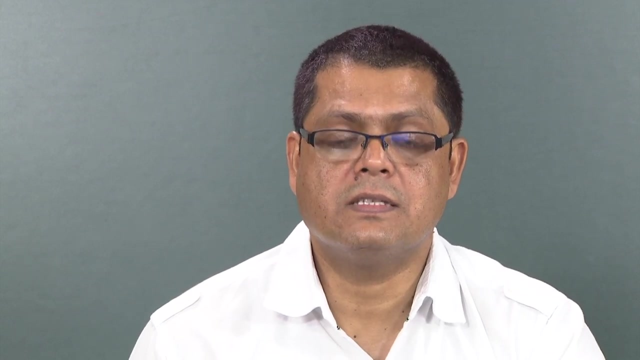 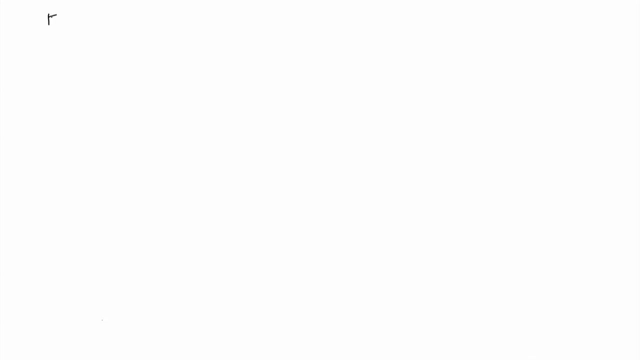 So we will start with discussing the entropy change for mixing of two ideal gases. So we will discuss mix entropy change for mixing of two ideal gases. So suppose initially we have a system having two containers and in one container bromine gas is there, in another container 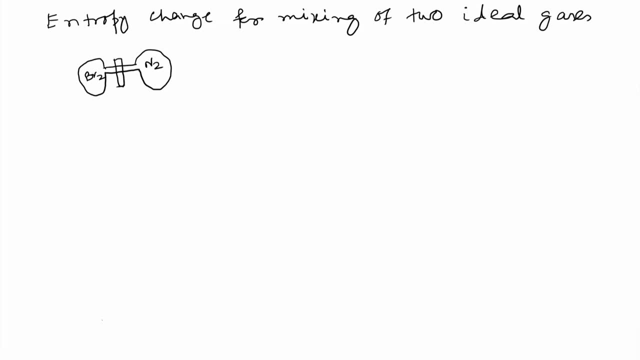 nitrogen gas is there. So this is our initial state And there is a stop quark between them. So if we remove the stop quark and they will mix. So here we have bromine plus nitrogen, Here also we have bromine plus nitrogen, And this is our final state. We are assuming here. 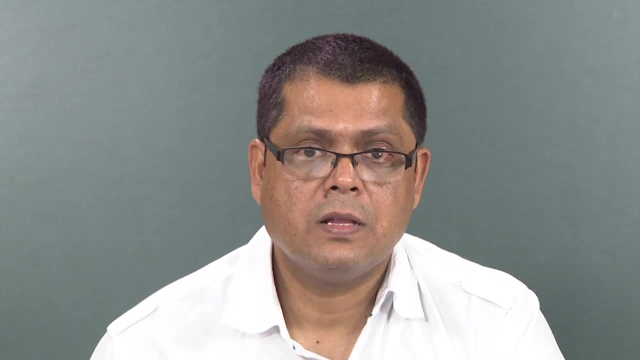 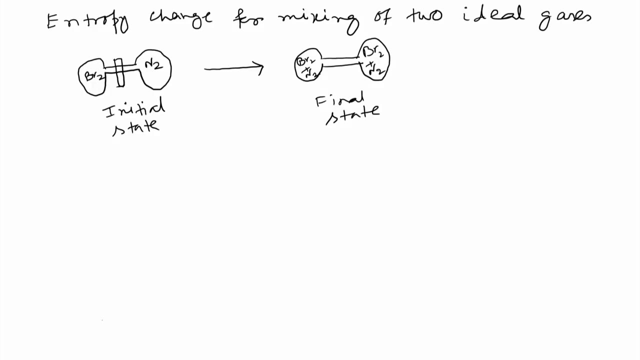 that both Because we know delta, S, Ln, V final by V initial. We already discussed that. Here Vn2 is the volume of this container and Vbr2 is the volume of this container, And nn2. here nn2 is the number of moles of. 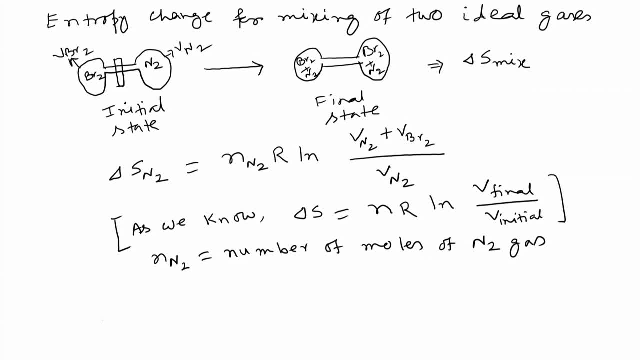 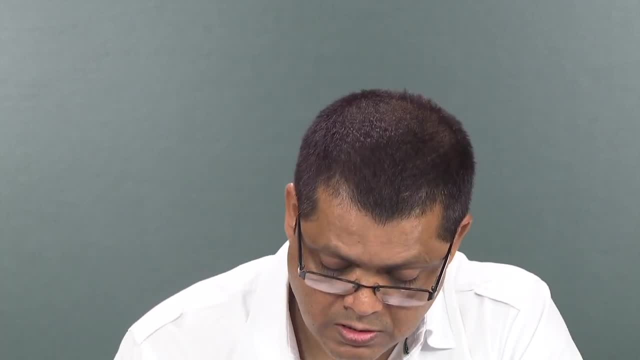 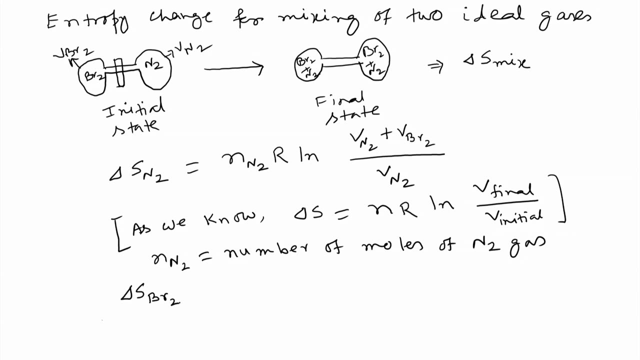 n2 gas. So this is the entropy change for nitrogen gas. What about entropy change for bromine gas? We say: this is delta Sp, hat 2.. In similar manner, we can write right A total entropy change. So what is the total entropy change? That is nothing but entropy. 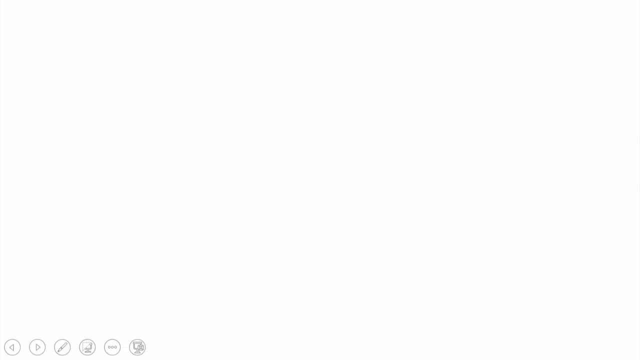 change for mixing. So delta S mix is nothing but delta S N2 plus delta S Br2, right, So we can write this: one is like: n into R ln, v into plus v b r 2. by v into plus n b r 2, R ln v into plus v b r 2. 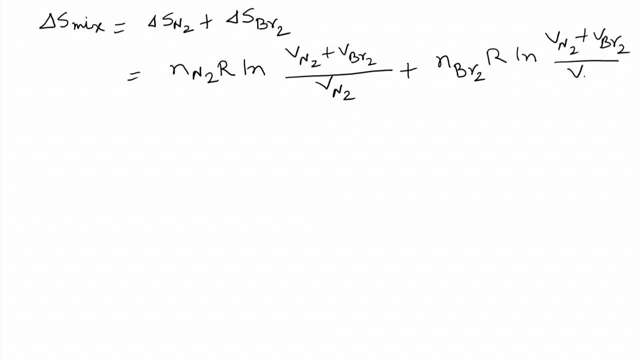 by v b r 2, very simple. Next, we can write like minus n into R ln v into, by minus n into by n b r 2, by v r 2 R. right Now, at constant temperature and pressure for ideal gas, we can write as N into R ln v, into plus n into plus n into plus n into. 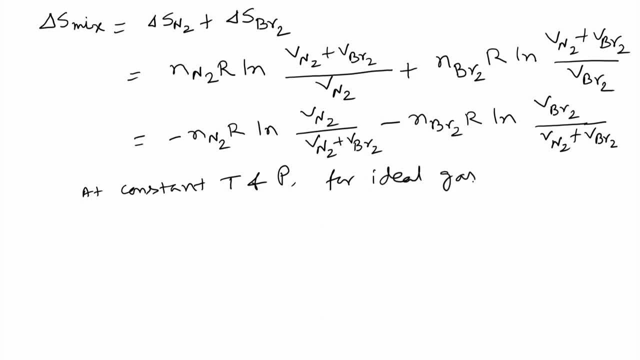 as volume is proportional to number of moles, right? So we can write: delta S makes x. Now we will just do some manipulation here- Where n is nothing but n, n, 2 plus n, b, f, 2 or total number of moles in the system. So 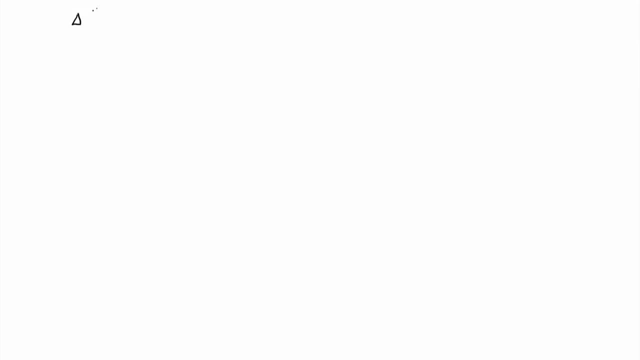 we can write: delta S makes S times n equal to minus f. 2 is equal to delta x n 2 plus n d 2, where x x n 2 is mole fraction of n 2. right, And this is nothing but your number of moles of n 2 by total number of. 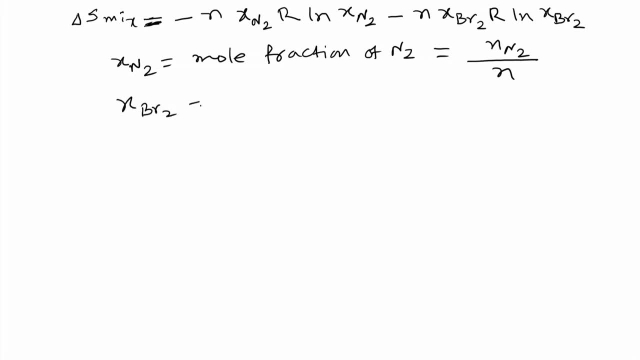 moles. Okay, Similarly, x B at 2 is the mole fraction of B at 2, and this is nothing but number of moles of B at 2 by total number of moles. So we can simplify this expression. or, in general: 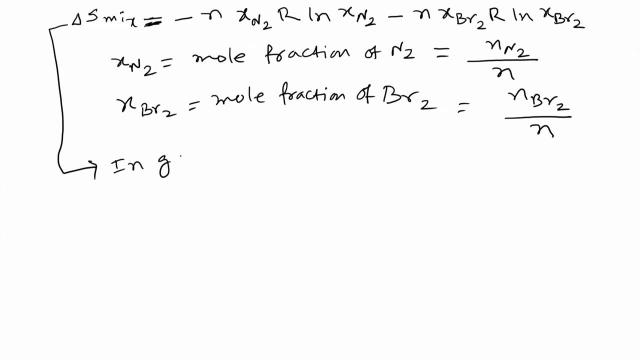 we can write. in general. we can write: delta S mixing is minus n? r sum over i, x i, ln, x i right, where x i is the mole fraction of ith species And in general is is is a fraction. ok, So x i, value of x i is or value of x i falls. 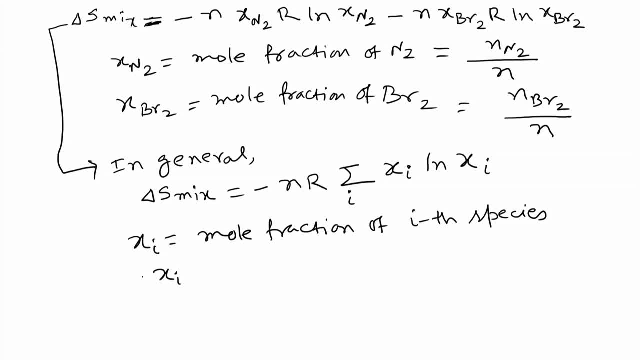 in between or mixing of entropy of mixing is positive, Or in other words, the mixing process is entropically. 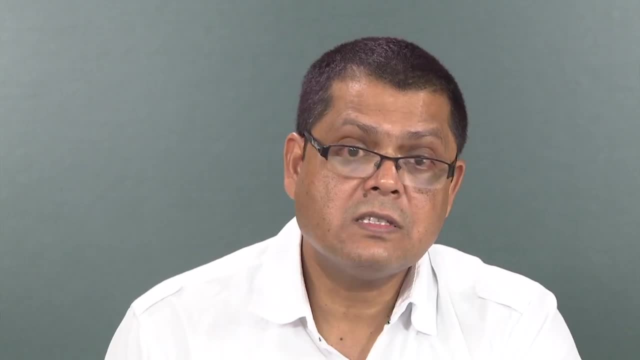 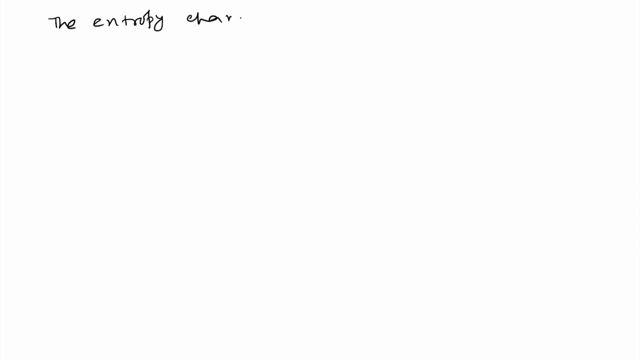 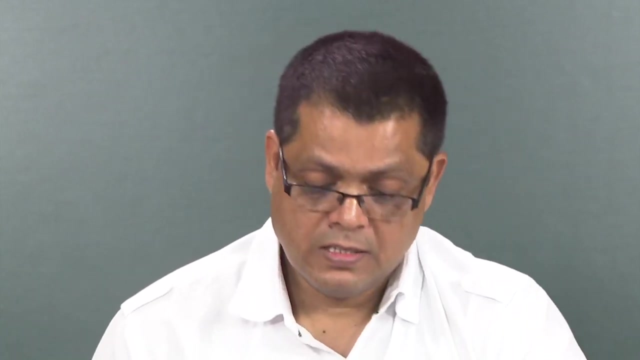 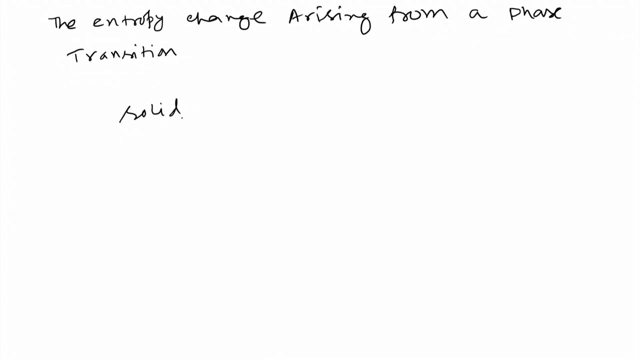 favorable. Next we discuss the entropy change arising from a phase transition. So next we will discuss what is the entropic change due to phase transition. okay, Now all phase transitions. suppose you have solid ice. When it melts it gives solid ice, solid. 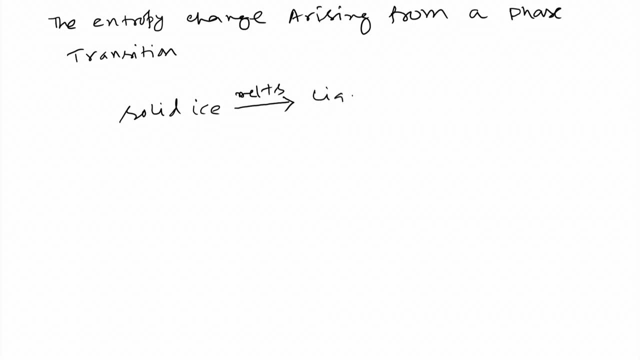 ice will melt, Okay Okay, Okay Okay. liquid water, and from there we get water vapor. right. So from solid to liquid, liquid to vapor, right. So when phase transition takes place. so these phase transitions are accompanied. 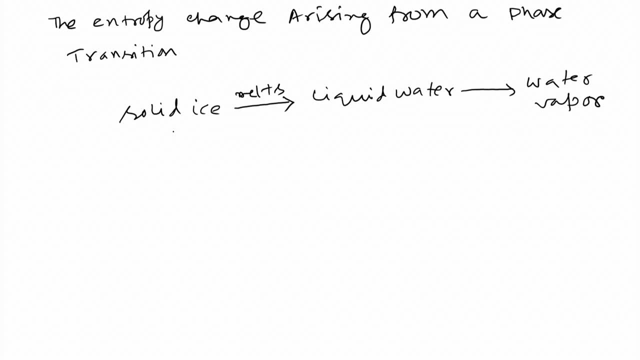 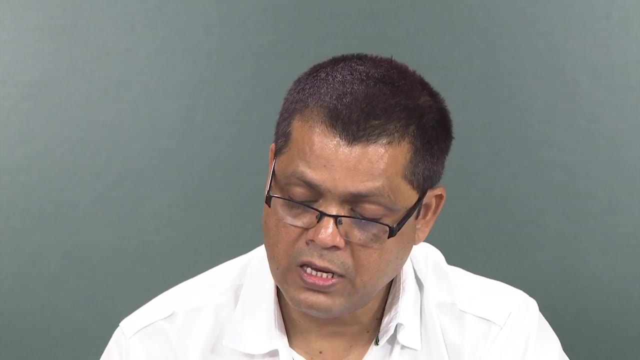 by change of entropy. okay, Because in case of solid ice, okay, the system is not that much chaotic. but when it melts and forms liquid water molecules are more chaotic. When it further boils, gives water vapor, it is further more chaotic water molecules. 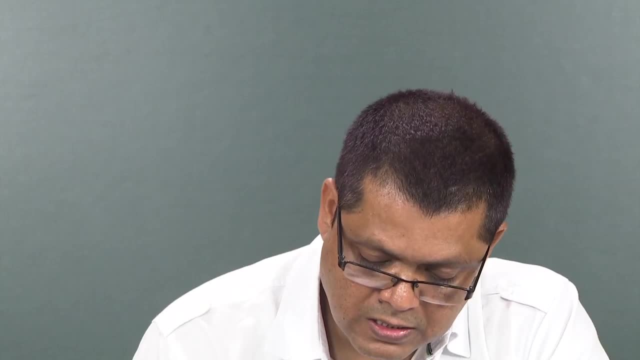 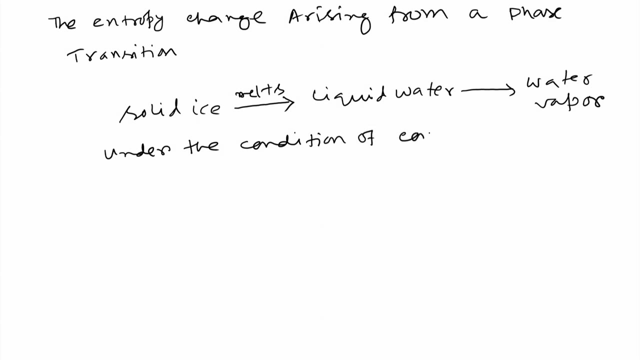 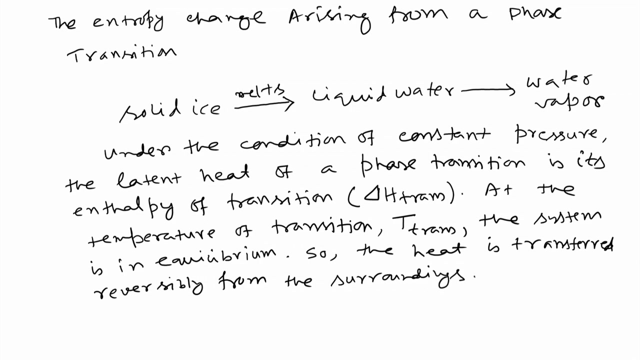 are okay. So under the condition of constant pressure. okay, The latent heat of of a phase transition is nothing but its enthalpy of of transition. okay, If we say delta H transition, it is nothing but delta H transition by T transition, right. 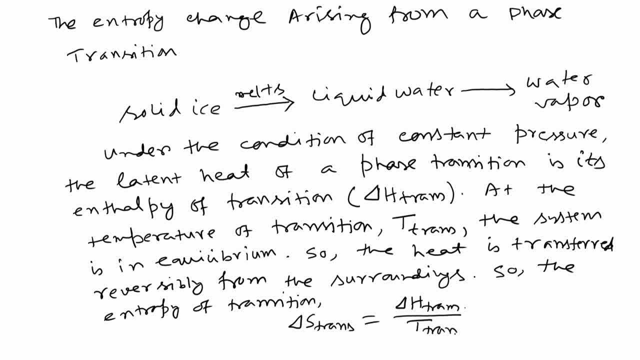 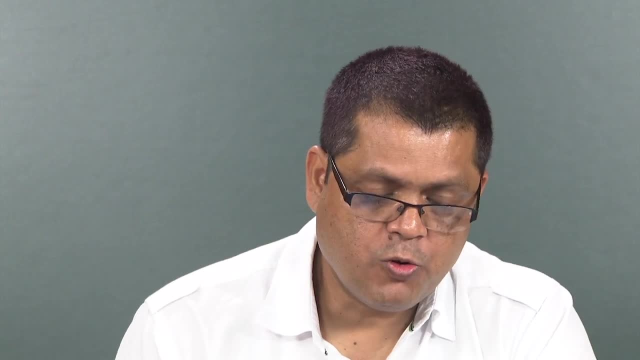 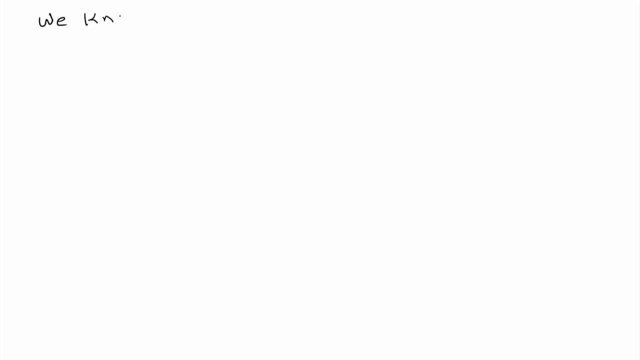 Now we will move. okay, we will move to something else, We will move to something else. So so far, what we discussed. We discussed that, or we know da system is greater than 0 for spontaneous process, right, But this is applicable for 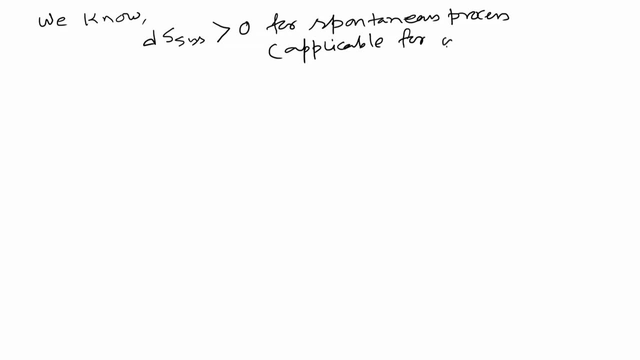 spontaneous isolated system only. So DS system change in entropy for the system greater than 0, for it says that the process is spontaneous process. but this condition is applicable only for isolated system, But in general means process can be isolated, the system can be isolated. 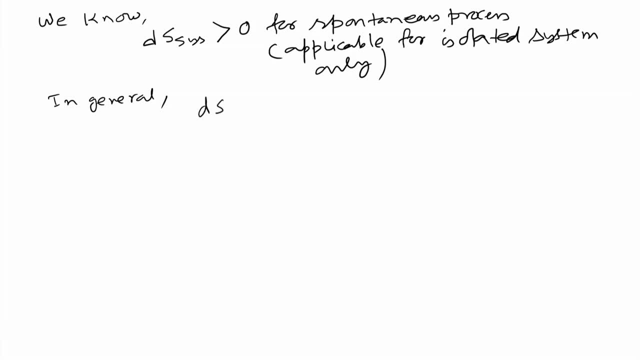 or non isolated. in general, DS total is nothing but DS universe equals to DS system 0.. 0.. So DS plus DS surroundings to be greater than 0 for spontaneous process. So in order to judge whether a system is a spontaneous or a non spontaneous process, we need to calculate. 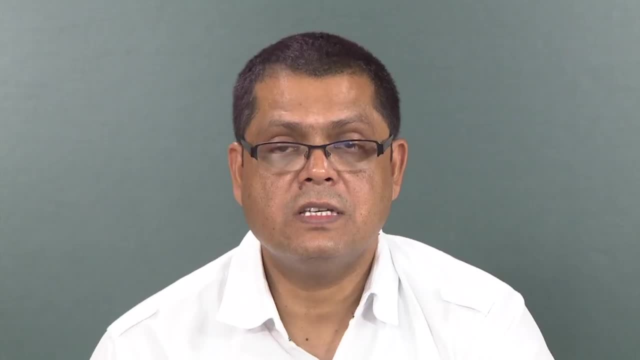 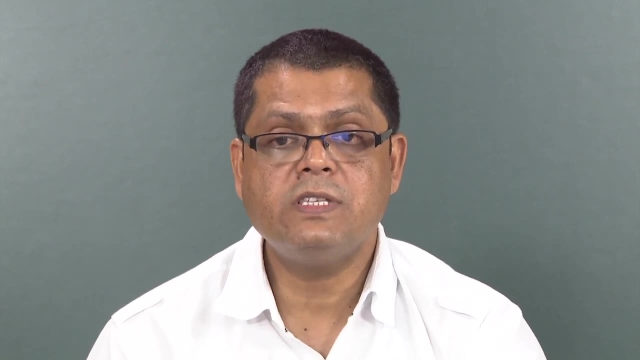 2 different quantities right- 1 is DS system, another is DS surroundings- will then sum them up and then we will calculate DS total or DS universe, and then we will check whether the value of this quantity is greater than 0 or not. then we can see that process is spontaneous. 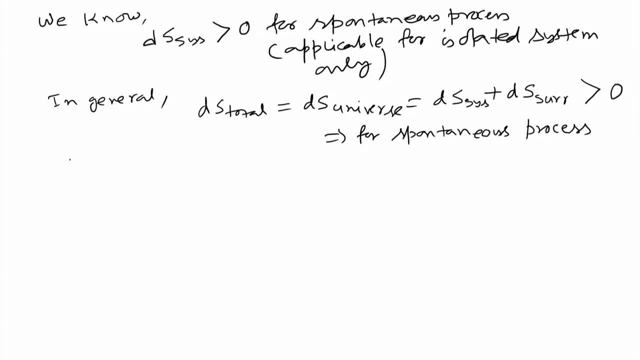 or not. ok, So in general, we need to calculate 0. 0.. 0. 0. 0. 0.. calculate two quantities, two quantities- ds system and ds surroundings, to judge or to examine whether the process is. so we need to calculate two different quantities ds system. 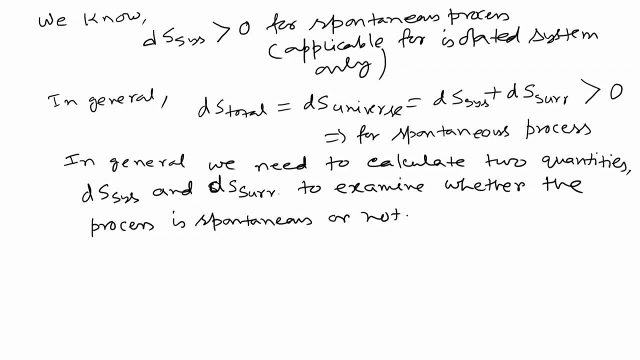 and ds surroundings. okay, in order to judge whether the process is spontaneous or not, It would be better if we can identify the spontaneity of any process by calculating only one parameter, right? So it would be better if we can identify the spontaneity of any process by calculating only one parameter right. 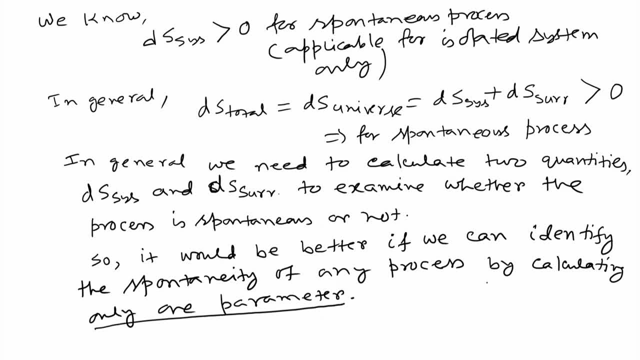 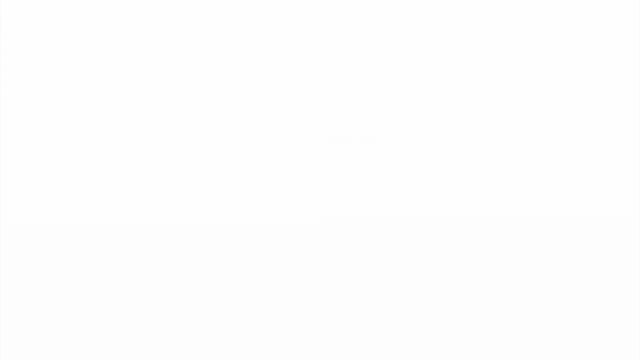 It would be better if we can identify the spontaneous count opening, which is of centimeter size, way more or less constant, right? It would have been further better if the parameter is a state function, right? So let us see whether we can have one single parameter that can tell us whether the process 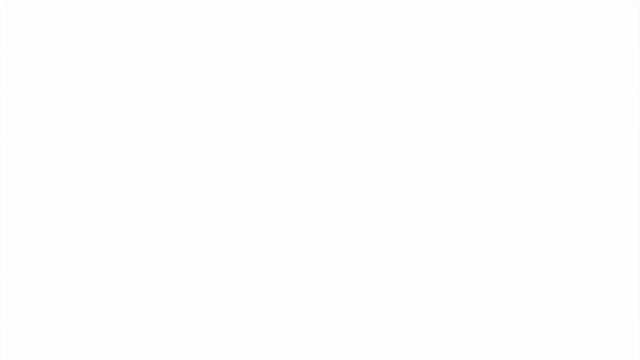 is spontaneous or not. So from Streisand, thermodynamics, from the scientific analysis development, a classic kids have done this kind of analysis, food problem today. So we were in NVT which there was very interesting kind of analysis, experiment, development. So what we have seen 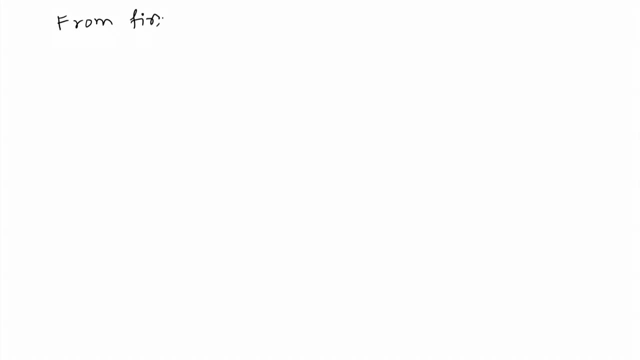 was the yelling, non sense descent. So in this you can see also we have that, we have there. So we know d? u is del q plus del w at constant volume, when volume is constant. at constant volume means no p v work. when volume is constant, there is no p v work. So d u is del q, right. 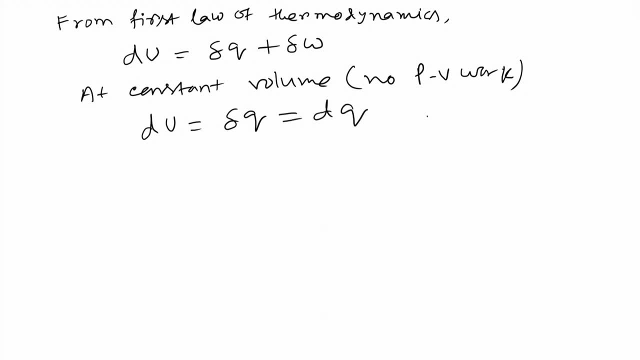 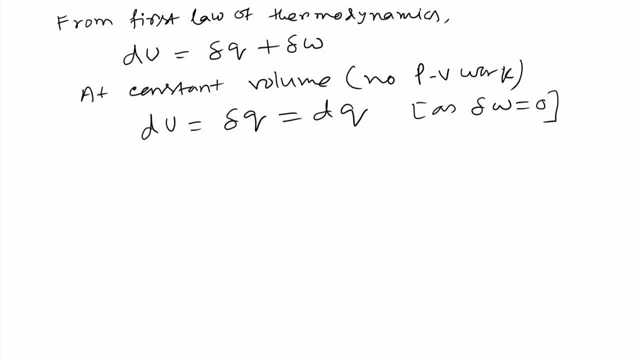 is 0.. Now in the in previous class we discussed our Clausius inequality and we know d s is greater than equal to del q by t. okay, So it says t d s is greater than equal to del. So we can write: du is less than equal to T ds. or we can write du minus T ds less than. 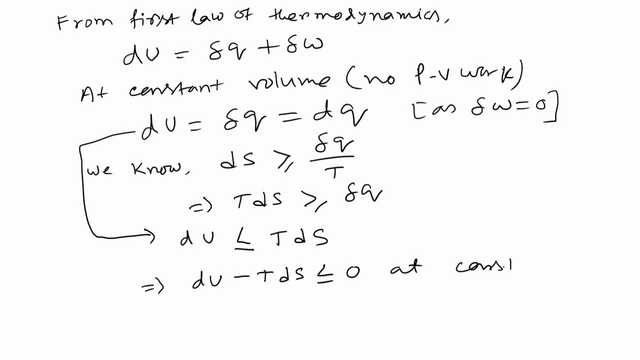 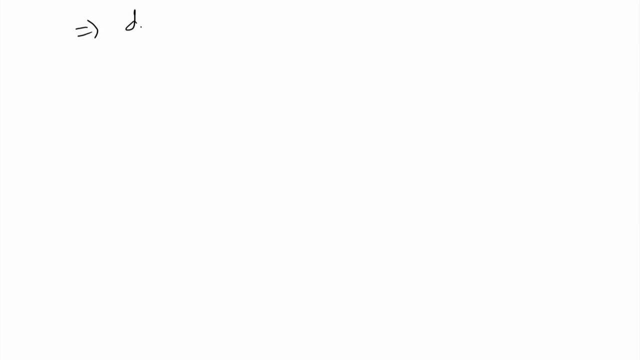 equal to 0 at constant volume. So we can further write: du minus T, ds less than equal to 0 at constant volume and temperature: okay, And this u minus Ts is known as Helmholtz free energy A. okay, So A at constant temperature. 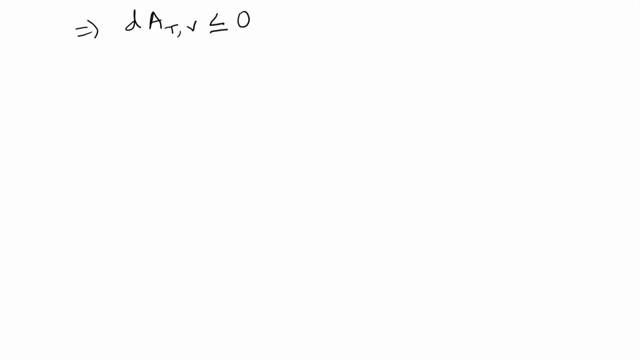 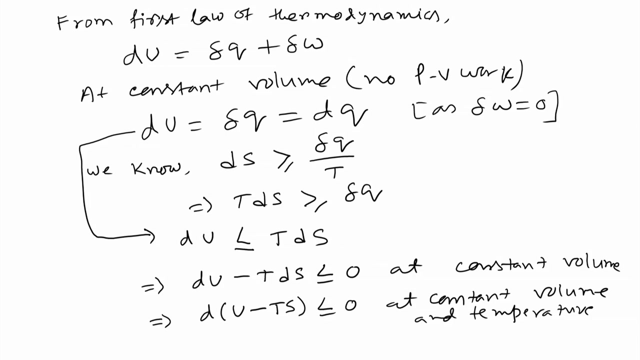 and volume less than equal to 0,. okay, So if you go back and check it, we use Clausius inequality right here. So this is the Clausius inequality we have used here. okay, So if you correlate with 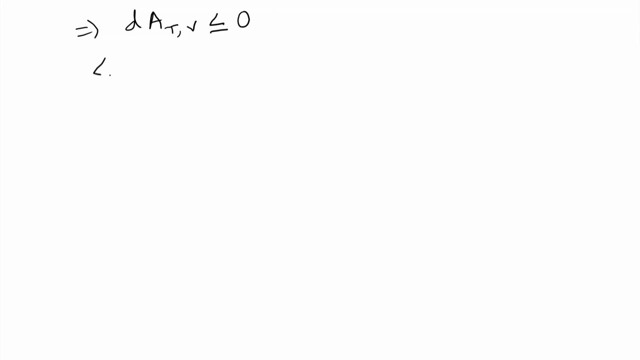 that and this expression- we can say this negative sign represents spontaneous process, Okay, And equal sign represents equilibrium, And A here we defined as u minus Ts, So A is known as Okay. So this is the equilibrium. 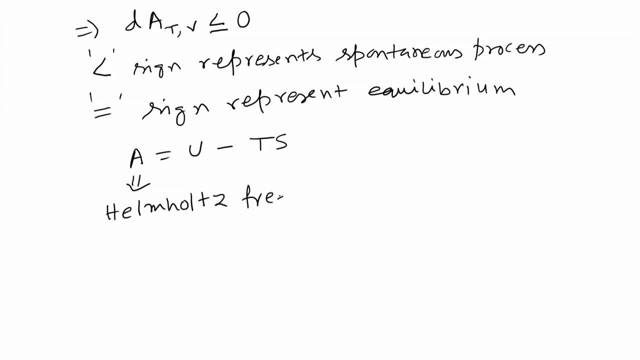 Okay, So this is the equilibrium. Okay, A is known as Helmholtz free energy, or sometimes Helmholtz free energy. okay, So this is the condition, this equation, if we say equation 1, this is the condition to check a process. 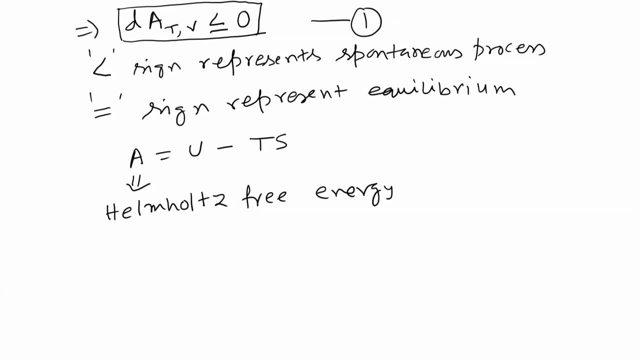 is spontaneous or not, when the process is being carried out at constant temperature and at constant volume. Okay, And this A is a state function. We can prove it. So, if we like, we plotted for entropy, if we plot a schematic diagram where we are plotting in Helmholtz free energy change versus 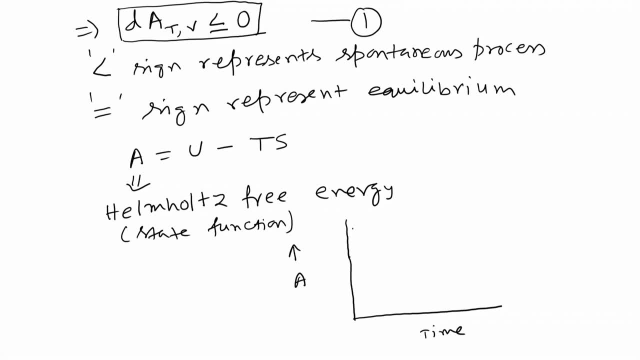 this. we get like this. So here, dA at constant temperature volume is less than 0 and dA dP equals to 0. Here, this is equilibrium and this is spontaneous process. Okay, So, this is the equilibrium and this is known as A minimum. Okay, So a process. when dA at 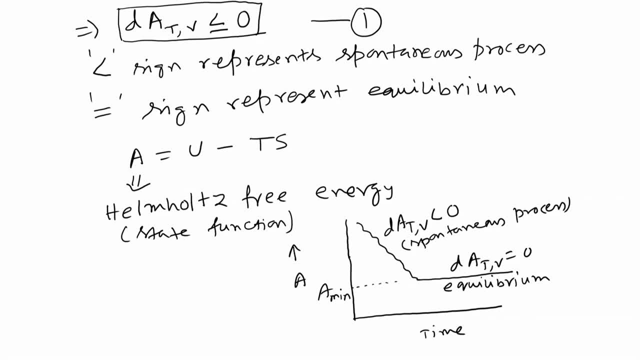 constant temperature and volume is greater than 0 cannot be a spontaneous one unless and until we do some work. Okay, And make the process spontaneous, Okay. So this is the equilibrium. Let us write after a while, so provide. Let us go again to the right We are levanting. 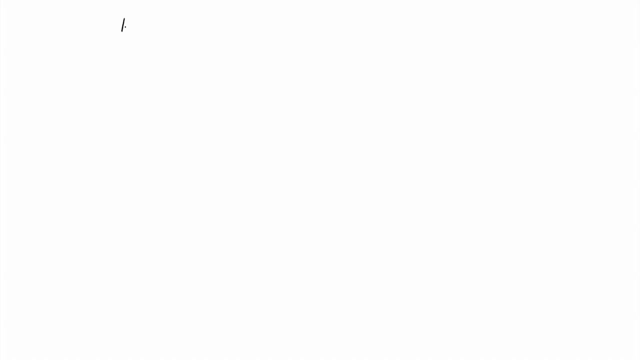 it. Okay. so we got A. is U minus T s, or we can write: del A equals to del U minus T, del s at constant T. okay, ワ. So this is the equilibrium and this is del A equals to del P, equals to dA. okay, So. 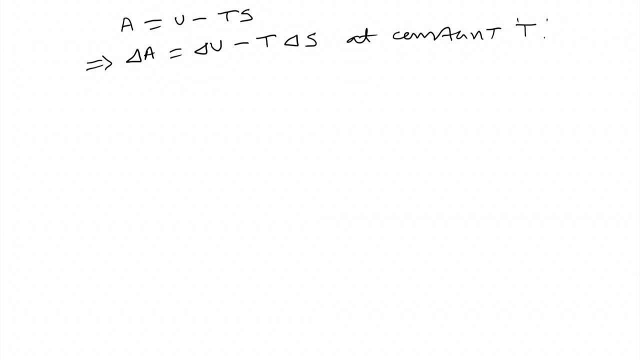 dS equals to dT. right, These are simple equations. Alright, We need a problem. We need a particular sı nä keeping constant temperature and47 degrees Celsius very easily. So what we and v? Now, if we look at this equation, equation 2 here, when delta u is less than 0, then 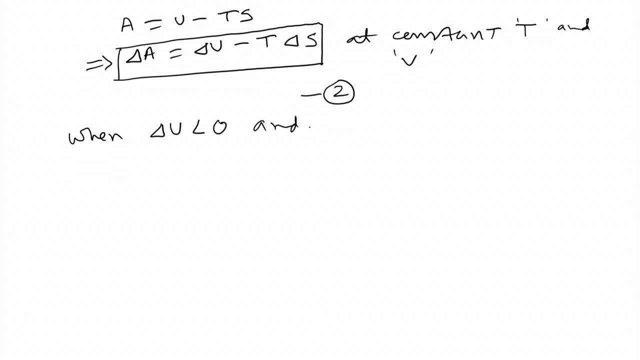 delta u and delta s is positive. when delta u is negative and delta s is positive, this makes delta a constant T v less than 0. So it makes the process spontaneous one okay. But if delta u and delta s, they have different sign okay. 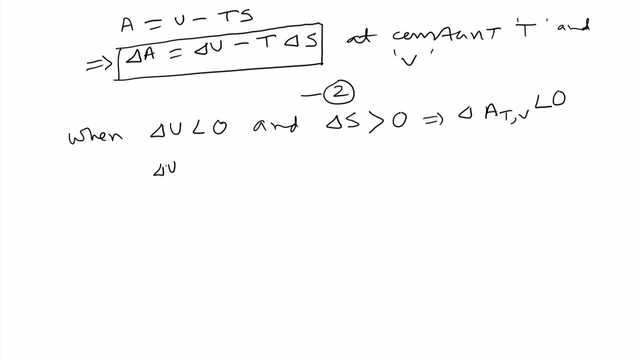 Suppose delta u is less than 0 and delta s is also less than 0, if they possess the same sign. okay, In that case, we need to, we need to examine the value of delta u and T, delta s. Okay, And then only we can judge whether the process is spontaneous one or not. okay, So, 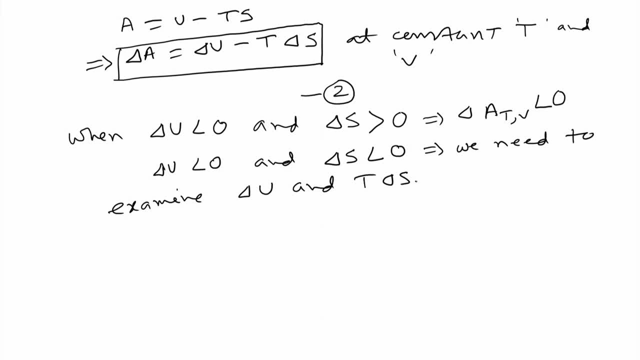 when delta u is negative and delta s is also negative. okay, we need to consider both the quantities When delta. is suppose, if delta u is positive, if delta u is positive and delta s is also negative, we have negative and then also negative wise. okay, we have. 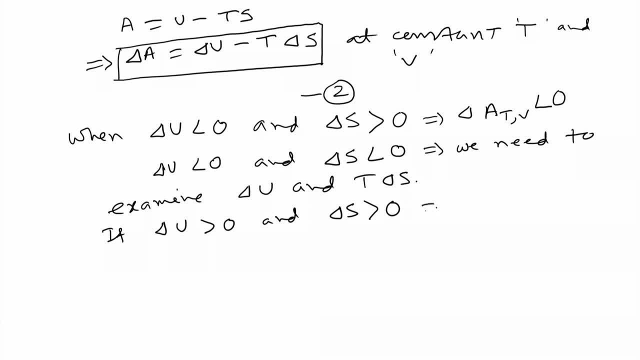 also positive. Okay, also positive. Then also we need to examine. we need to examine both delta u and T delta s terms, Both the terms we need to consider, and then only we can judge whether the process is spontaneous or what spontaneous one or not. 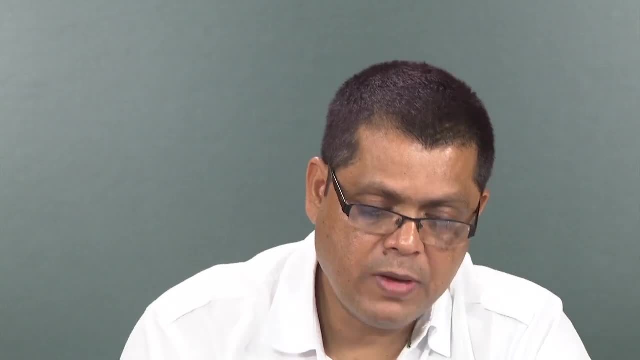 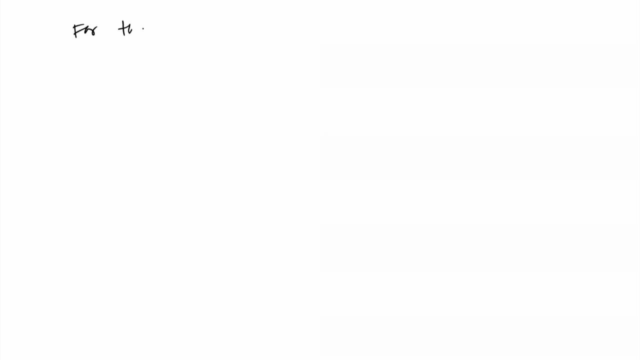 Now, if we think about the entropy of mixing- the experiment we carried out for the mixing of bromine and nitrogen gas that we discussed just now- We know delta is mixing is minus nr, Right, Sum over i, xi, ln, xi, Right. And this mixing process, for this mixing process, delta u is 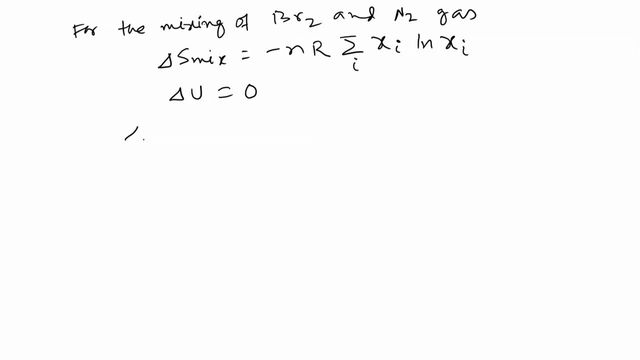 0. Right, So what is delta a there? So delta a mix is nothing but n? r T sum over i, xi, ln, xi. And since xi is a fraction, same mole fraction is a fraction, Right, Right. And since xi is a fraction of quantity, we can say: delta a mix is less than 0. Okay, 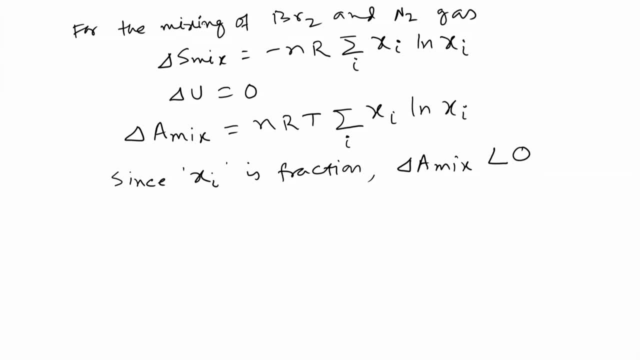 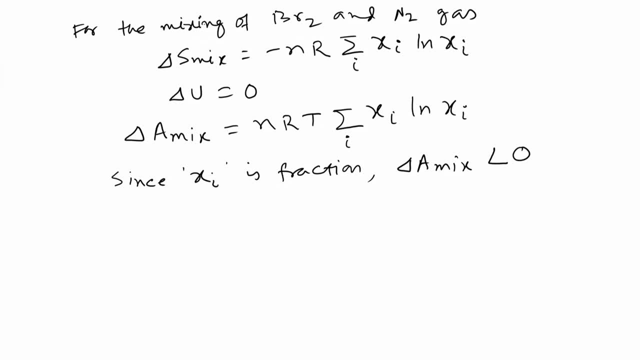 At constant temperature and pressure. So we need to have a parameter, or rather a state function. by examining that state function at constant temperature and pressure process, If we can say the process is spontaneous, 1 or not, Right, So that is how the Gibbs free. 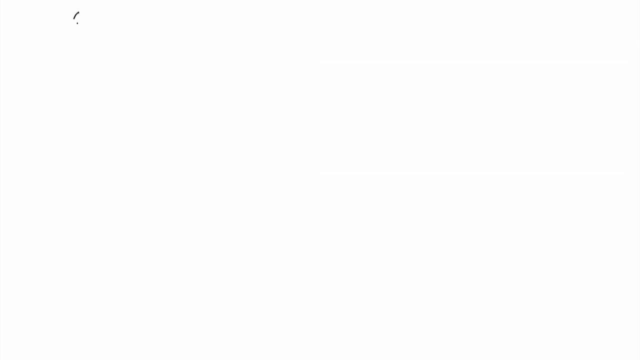 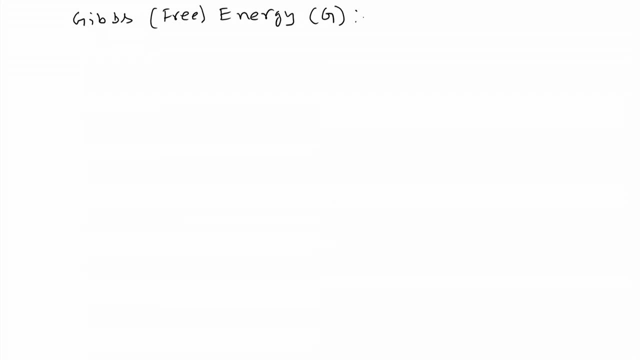 have g. why Helmholtz? free energy is not sufficient because most of the, or since most of the reactions right, Right, These are because the reactions occur at constant T and P. So it would be better if we define a state function which helps in determining the spontaneity of a process at 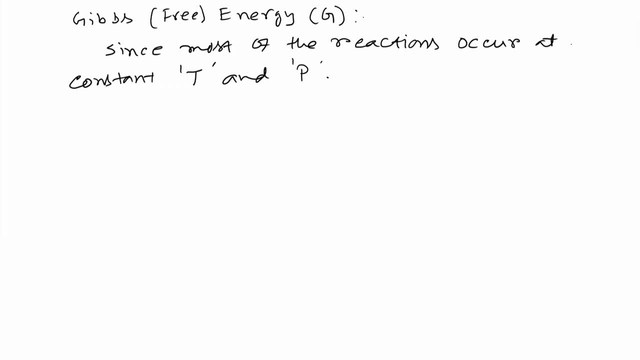 constant temperature and pressure. So we will define that quantity now. So we know d e o is del q plus del w. Remember, here pressure is constant, unlike for the case of Hilmuth- free energy- where volume was constant. So we could able to make del w 0, but here del 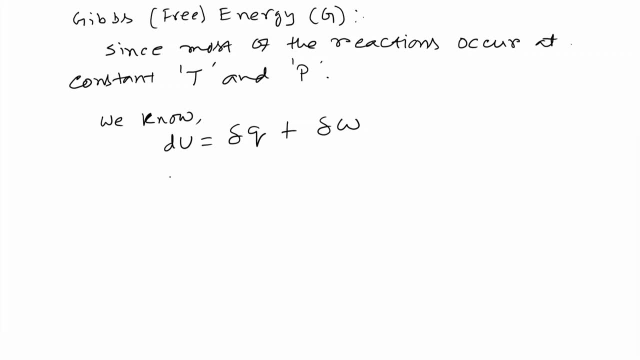 w is not 0.. So now we know again: del q by T or d s is greater than equal to del q by T, or in other words, T d s is greater than or equal to del q. So we write: d e o is greater than or equal to del q by T, or in other words, T d s is greater. 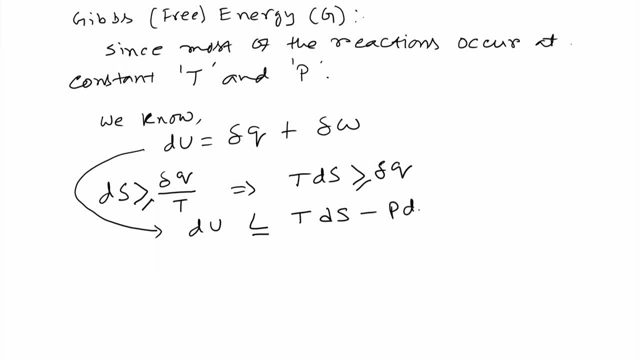 than or equal to del q by T. So since del w is not 0 here, So del w is nothing but P d, v. So we can write: d e o is equal to del w by T, or in other words T d s is greater. 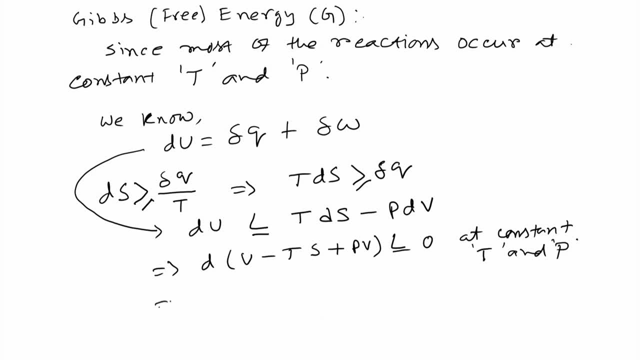 than or equal to del w by T, So at constant temperature and pressure. this is the expression, and we know u plus P, v is nothing but enthalpy. So we can write d H minus T s is less than equal to 0. or we can write d g at constant temperature and pressure, less than or equal. 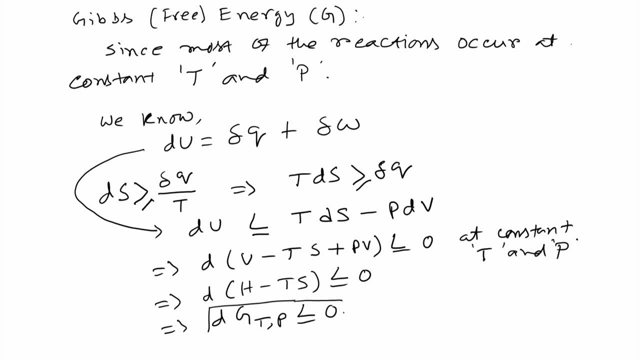 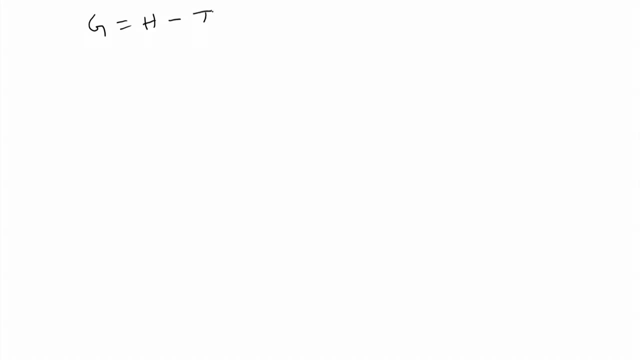 to 0.. This is the expression d. g at constant temperature and pressure less than equals to 0 is the continuous conditions for spontaneity of. So here g, so g. here is nothing but h minus Ts. okay, Next we will discuss how g varies. 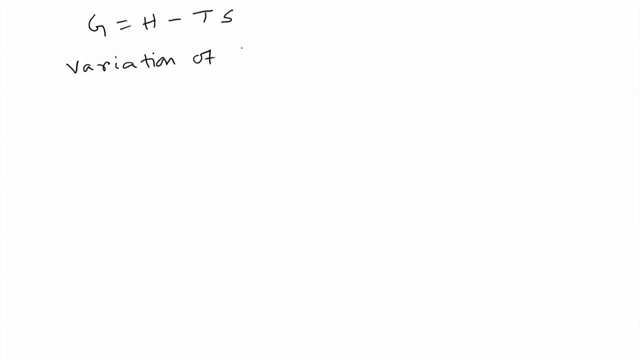 with temperature and pressure. So variation of Gibbs free energy with temperature and pressure. So this thing we will discuss now. This is very important expression. we will arrive, two very important expression. we will arrive. okay, if we consider the variation of Gibbs free energy with temperature and pressure. okay, 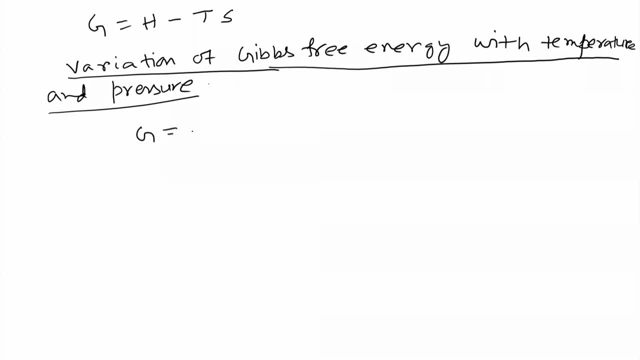 So we know g is nothing but h minus Ts. So we can write dg S dh minus T, ds minus S dt. Now h is u plus P dv, So dh is nothing but du plus P dv plus V dp, right? So if you? 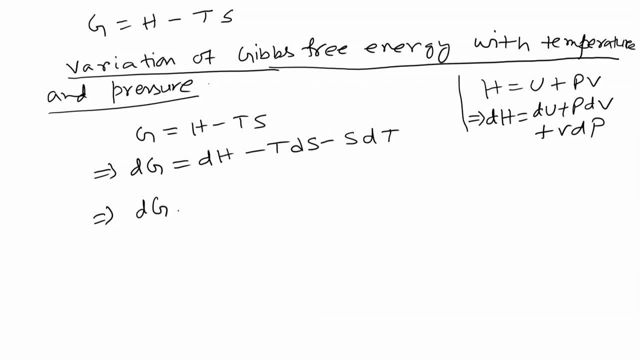 substitute the value of dh, here we get dg is du plus P dv, plus V dp, minus T ds plus minus S dt. Next is: what is du plus P dv? So du plus P dv? this term is nothing but dq, and T ds also is nothing but dq, okay. So we write: dg is nothing but dq plus V dp minus. 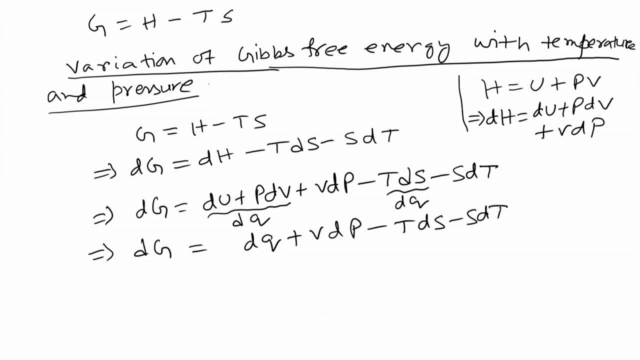 T ds minus S dt. okay, And this T? ds also is nothing but dq, or rather del Q. here we cannot write dq, here we write del Q. okay, So we write: dg is V? dp minus S? dt. So this is a very, very important expression. 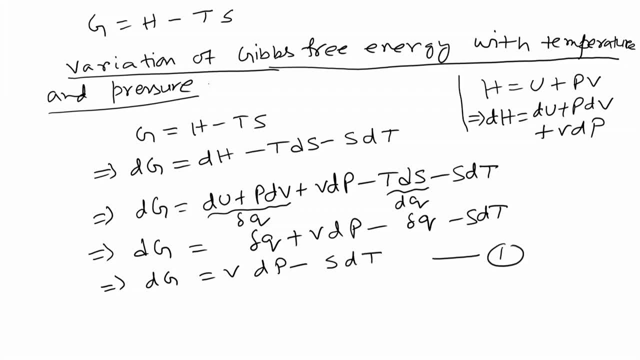 Okay, So this is a very, very important expression. okay, So this is your next example. You have to have the same equation right. You have to expression Why We will see now. So we get dG equals to V dP minus H dT From there. 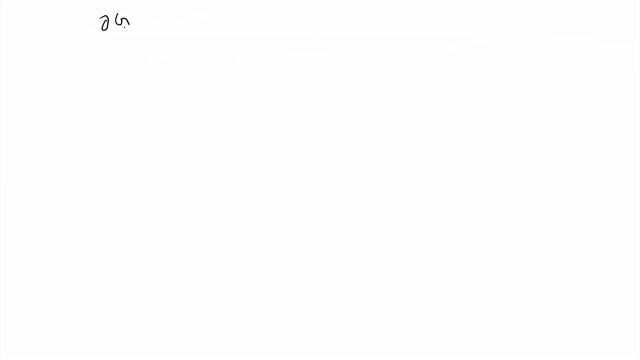 we can write del G by del P at constant temperature gives volume. So if we vary G with pressure at constant temperature, we get volume. So this is our equation. suppose this is our equation 2 here. and del G by del T at constant pressure, we write minus H. So this is our. 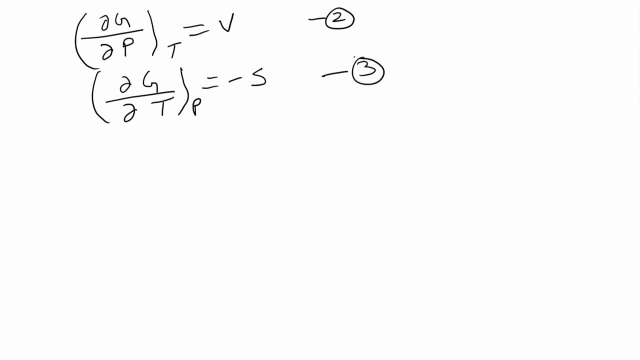 equation 3.. And these two expressions, these two expressions are very, very important. We need to remember those two expressions. okay, Now, if we consider First, we will consider this expression, expression 3,. okay, So we will consider expression. 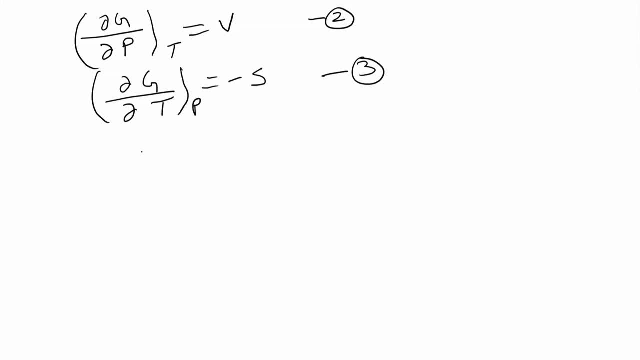 3 here. okay, So we get. this is expression 3, okay. Now, if we plot G versus temperature in Kelvin, right Expression 3 says: variation of Gibbs: free energy with temperature at constant pressure. So this is at constant pressure. 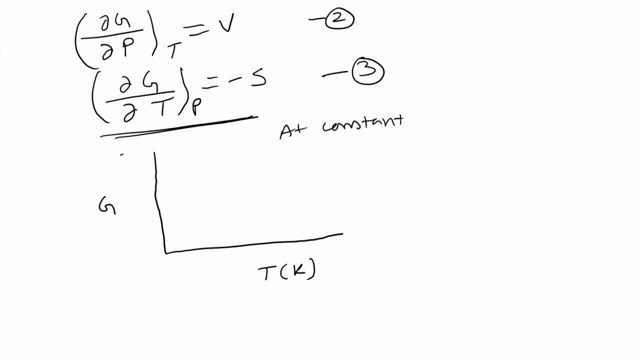 Okay, So in expression 3, if we look at expression 3 here, we get that the slope of the curve is negative, right? because absolute entropy is a positive quantity. So the slope of G, G versus t plot will be having negative slope. So the plot of G versus t will be having 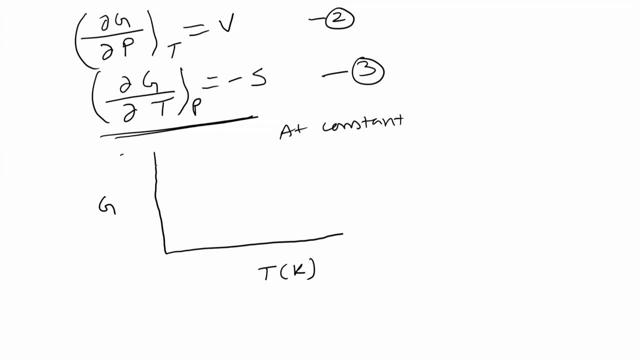 negative slope. So we get like this: If you look at the figure carefully, what you observe? You observe that the slope is different up to this point, Again, from this point. to this point after this point, the slope is also different here. So this is known as melting temperature. 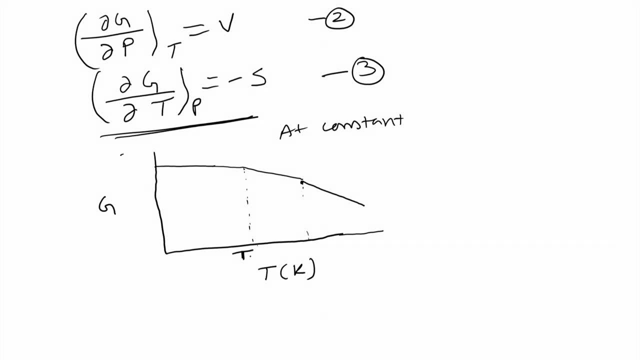 Okay, Melting point. we can say: So this is melting point, This point is melting point And this is boiling point Why the slopes are different here. So the slopes are different here because S? Okay, Because gas absolute entropy for gas molecule is much, much higher than S liquid, which is 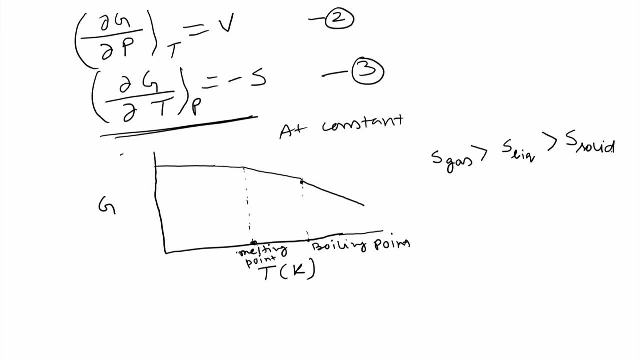 greater than S- solid. Okay, That is why we get different slopes here. So this region is our solid region. This is liquid region. This is solid region. This is liquid region. Okay. So this is at constant pressure. Okay, When pressure is constant, we get this kind of. 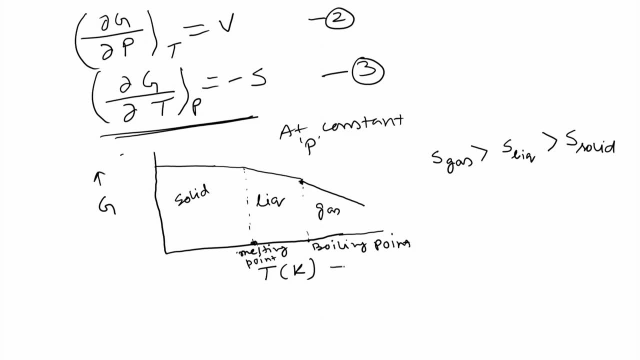 plot, If we plot G versus t, Now, few important expressions. now we will consider another expression, Right, That expression 2.. So from expression 2 or equation 2, we can write: dG equals to Vdp, Okay, And G1 to G2 limits are equal to Vdp, Okay. So we can write this. So we can. 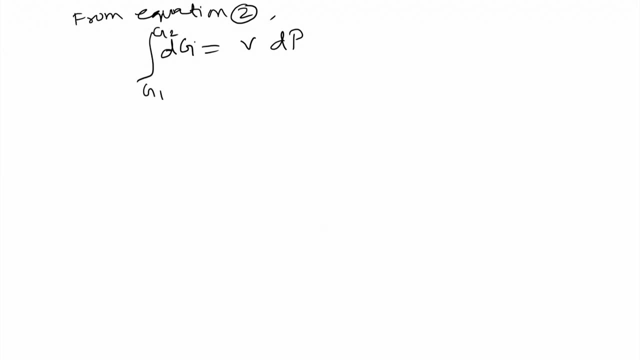 write this, Okay. Okay, So we can write this. Okay, So we can write this. So here and here, P1 to P2.. Okay, So for ideal gas, V is nothing but A nRT by P, So we can write: del, G is nothing but G2 minus G1 is A nRT ln P2 by P1. 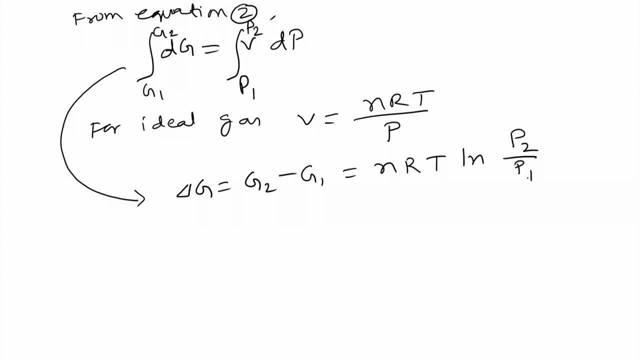 Okay, Okay, Or we can further write: del G is nothing but A nRT, ln, V1 by V2, since P is inversely proportional to V at constant t and n. Okay, So we get another good expression, another nice expression for calculating delta G. 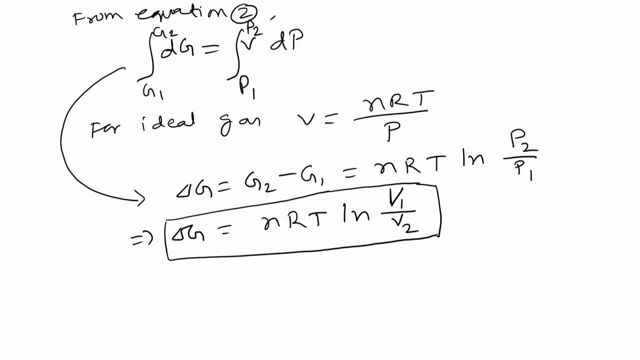 Okay, So so far what we got, if we summarize what we have discussed so far, we have dU is T, dS, or rather we can write del Q if the process is reversible, one del Q plus del W reversible. Okay. 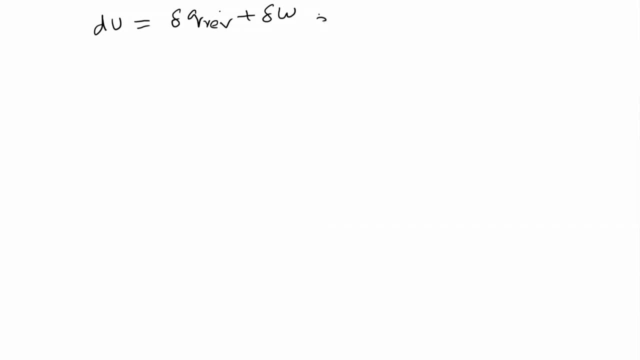 Okay, So we can write: dU is del Q plus del W, and we can write this one as T, dS minus P, dV. Okay, Okay, And from here we can write del U by del S at constant volume is T and del U by del V. 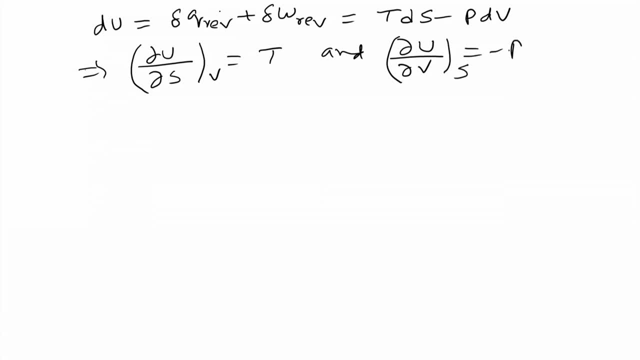 at constant S is minus P. Okay, So from here we get the definition of absolute absolute temperature. Okay, If we vary, if we calculate del U by del S at constant V, we get temperature. Now we also got dH. dH is nothing but dU. 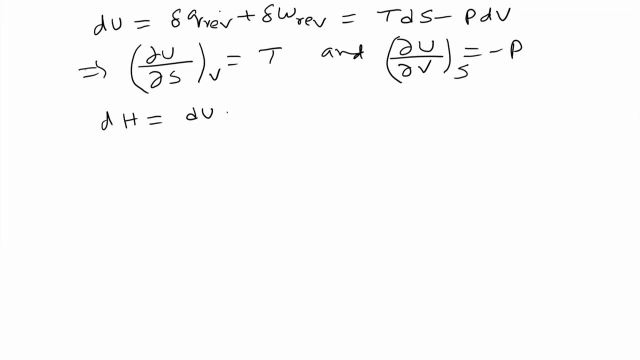 Okay, Okay, Okay, Okay, Okay. So del U by del S plus P dV plus V dP, Okay So dU plus P dV is nothing but del Q plus V dP, and del Q is nothing but T dS plus V dP. 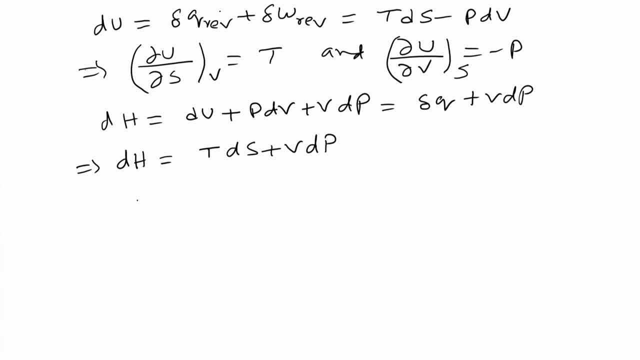 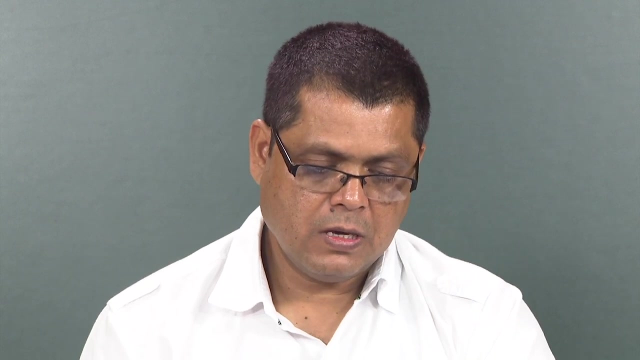 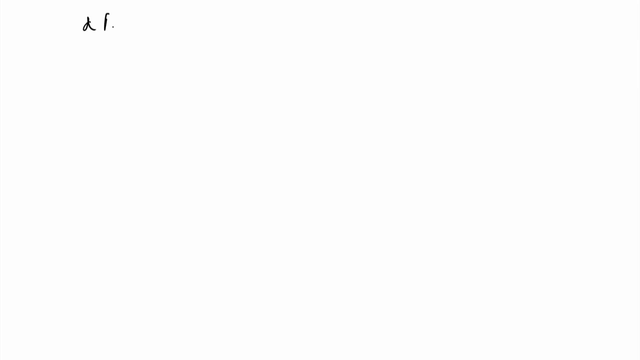 Okay, Okay. So if we do the way we did it before- Okay, we did it before- we get: del H by del S at constant pressure is T, and del H by del P at constant S is V. Then we have A, so we know A. so dA is dU minus T, dS minus S, dT. 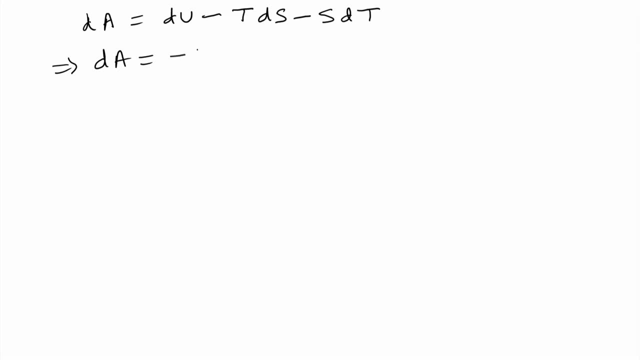 So if we further simplify this one you get dU is minus P dV minus S dT, Because this dU you can further write like T dS minus P dV, minus T dS minus S dT. This is your del Q and this is your del W. So from this expression, dA equals to minus P dV, minus. 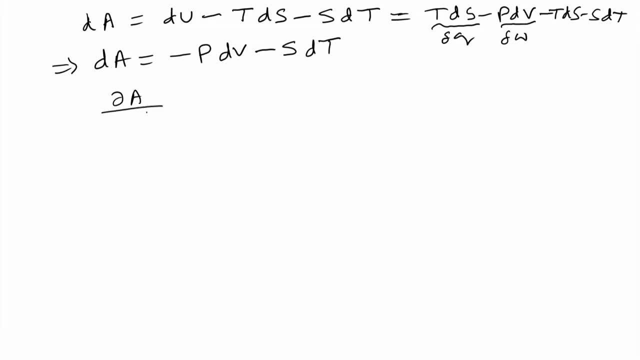 S, dT. We can write: Del A by del V at constant temperature is minus P, and del A by del T at constant V is minus S. And lastly, we know dG is dH minus S, dT. So we find B by del W, D, C minus T, dS and H. we know dU plus P, dV plus P, dP minus S, dT.